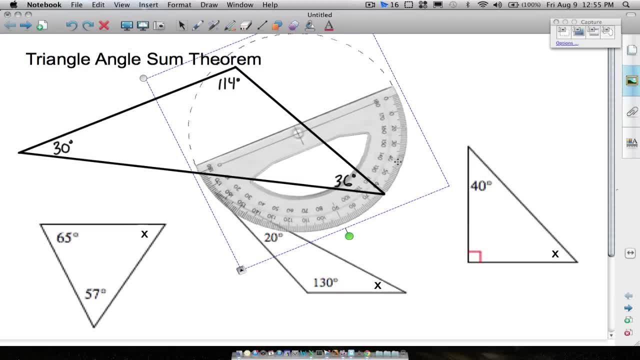 Now, why did I do all this? Well, if we look at these three angles which we have measured, if we add these together, 114 plus 36 plus 30,, 4 and 6 is 10, put down our zero, carry our 1,, 3,, 6,, 7,, 8, and then there's 1. 180 degrees. There's your triangle angle sum theorem. 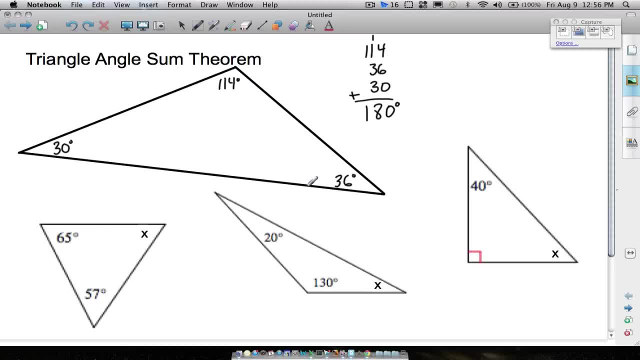 I drew a totally random triangle. If we add up the three degrees inside of it- this is your rule or your thing that you want to remember about three angles in a triangle- The three angles will always add to give you 180 degrees. That's what the triangle angle sum theorem is. 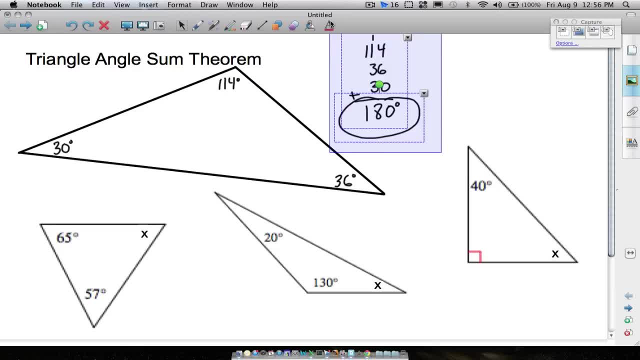 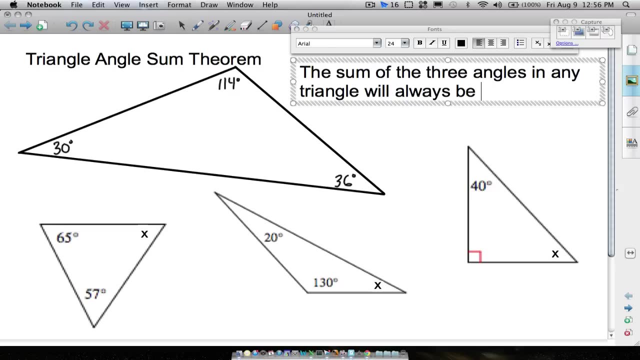 So let's write that down. The sum of the three angles in any triangle will always be 180 degrees. With that in mind, these three examples down here, we're given two angles. We need to find the third angle. So what we can do, you can either add these two together and then subtract that number from 180,. 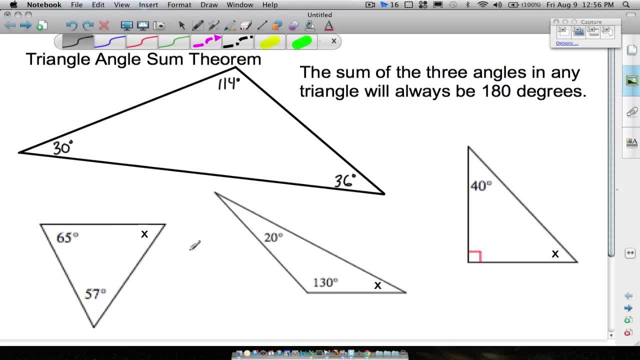 or you could take 180 minus 65 minus 57.. It's entirely up to you how you want to do that. So take your 65 and 57, add those two together. If you add 65 plus 57, you get 122. 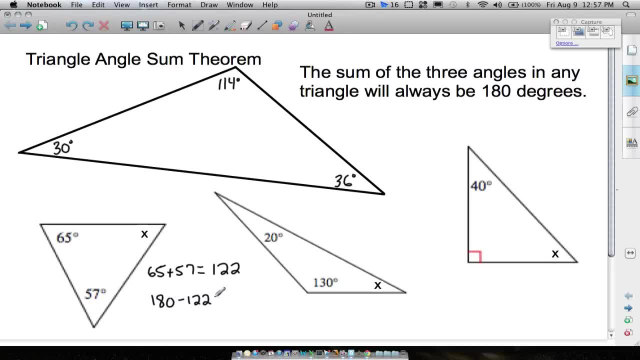 And then if we take 180 degrees minus 122, because we need that third angle right there- subtracting that you get 58 degrees. So therefore x is going to be equal to 58 degrees here, And you can double check your work. 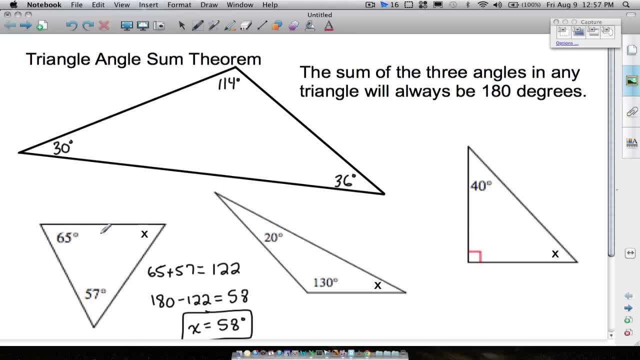 What you can do is you can add all three of these numbers back up. add them back together: 58 plus 65 plus 57 is equal to 180 degrees. So that's our solution to this problem. here Now this second triangle: same idea. 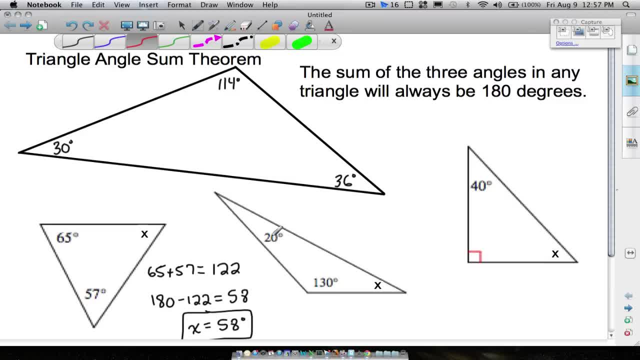 We can add these two angles together: 130 plus 20 is going to be 150.. If we take 180 minus 150, you get 30 degrees. So therefore, x is equal to 30 degrees And this one right here.